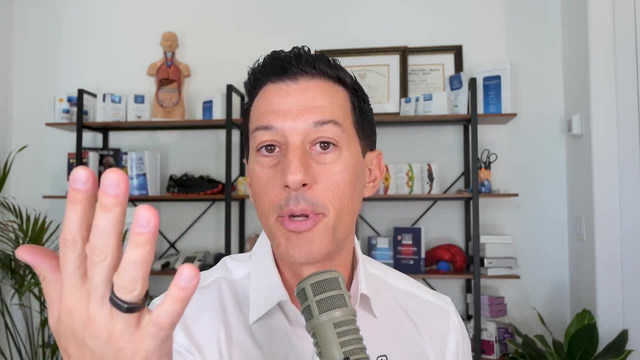 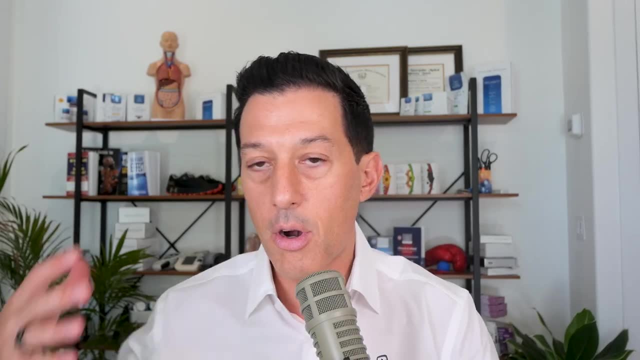 arsenic, mercury, cadmium and aluminum. All right, So we're going to talk about some of those today. So those are the ones that we want to watch out for, and they don't just affect our nervous system, eyesight or give us headaches or blood sugar issues. They actually cause an inflammatory 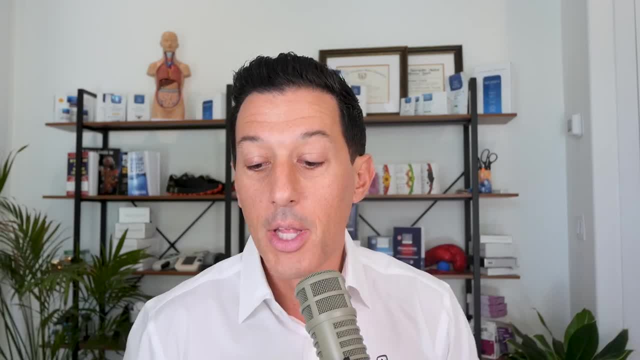 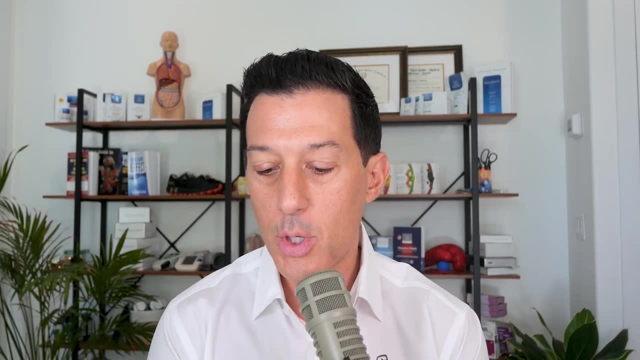 response when they are consumed and digested. Now, the main place that you're going to find these heavy metals is typically from water-based contamination, So I'm going to give you a quick rundown here as well. So aluminum is, when we run a minerals and metals test, the most pervasive. 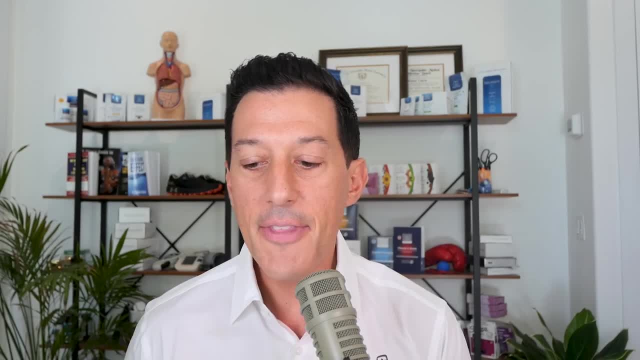 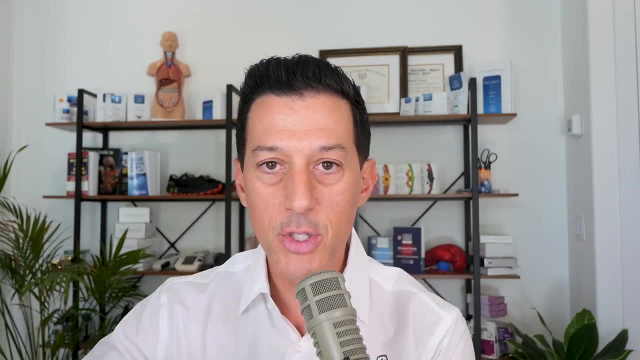 meaning the thing that we see the most is always aluminum. It's typically what we see And that's because it's in aluminum. well, let's talk about this: deodorants. It's in aluminum pans, aluminum spatulas when you scrape the pan, aluminum foil- many other factors- but it's also used in drinking. 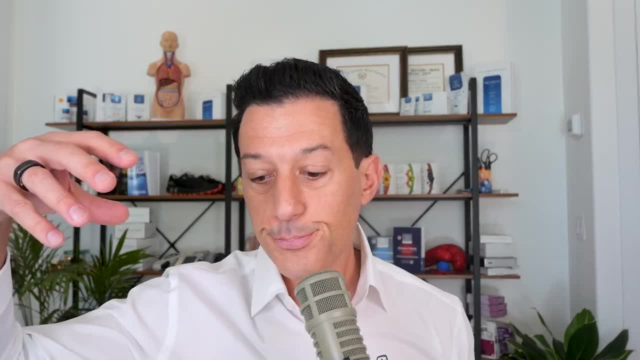 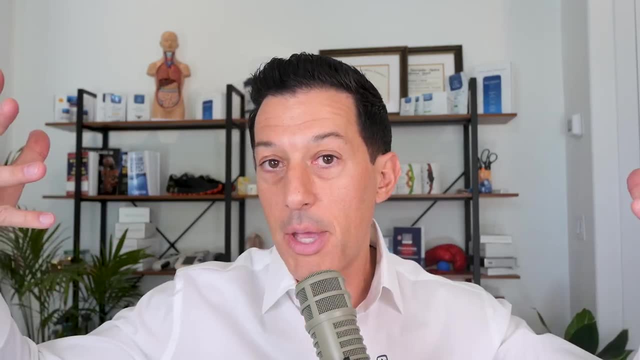 water and tap water, And that's because they'll add aluminum as what's called a surfactant, And essentially what it's going to do is it's going to attach itself to other minerals, potentially, and it's going to pull them down to the bottom of the tank. Now, some aluminum is still left. 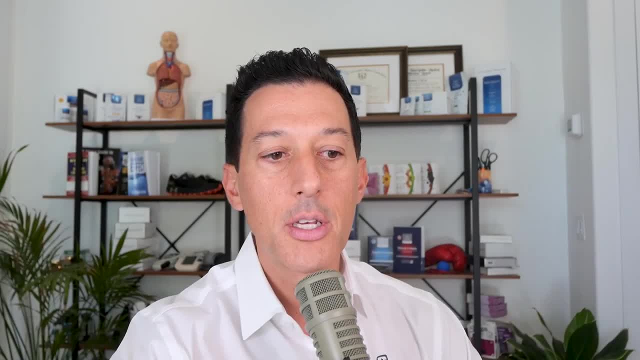 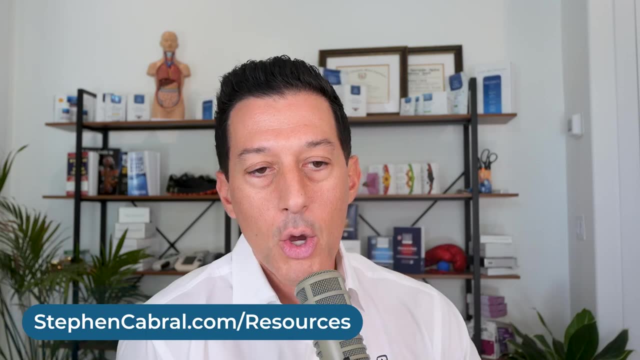 but it gives you clear drinking water, And so that's a lot of times why you're using aluminum in water Again. that's why we always recommend water filters. All the water filters and the companies I recommend are at stephencabralcom. forward slash resources, but that's a big one, Okay. 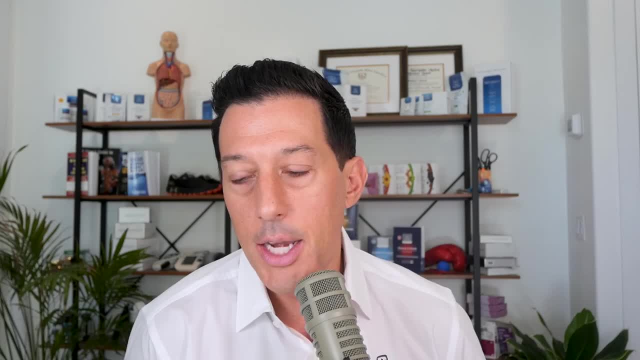 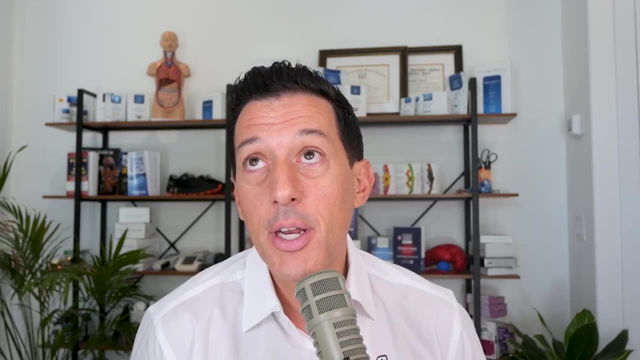 Then there's also arsenic. Arsenic is added. I again like not a good idea, but it's added to water in many parts of the world. You can see it in pesticides and a lot of people talk about it in the soil. Yes, it's in the soil, but oftentimes it's because it's from contaminated water. 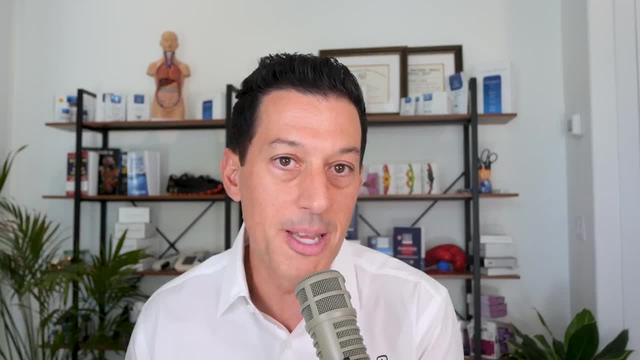 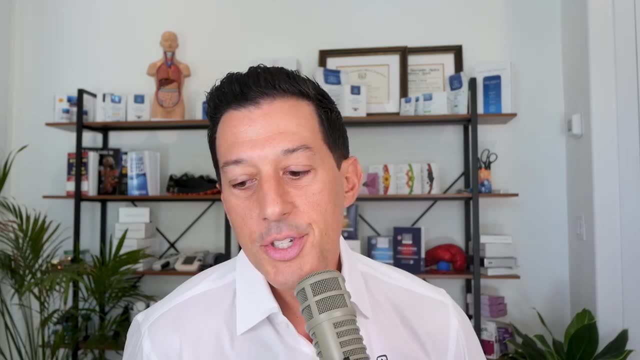 And then it gets in like rice patches, because rice grows basically in water, water and soil And that's why the rice can sometimes have higher levels of arsenic. So important to just make sure that you're consuming a low arsenic rice If you're having rice. 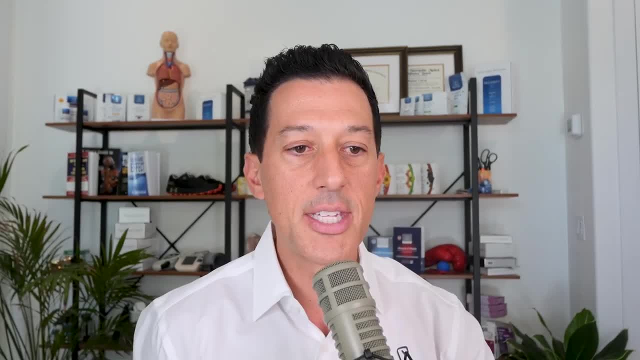 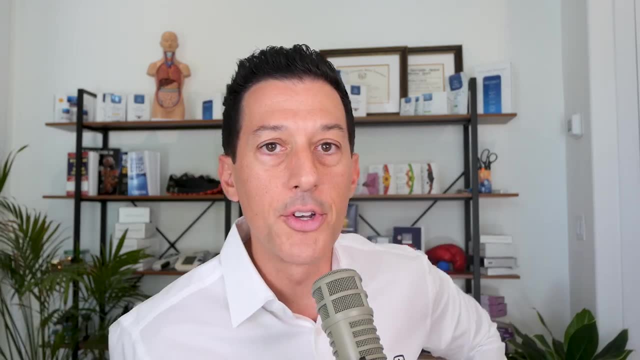 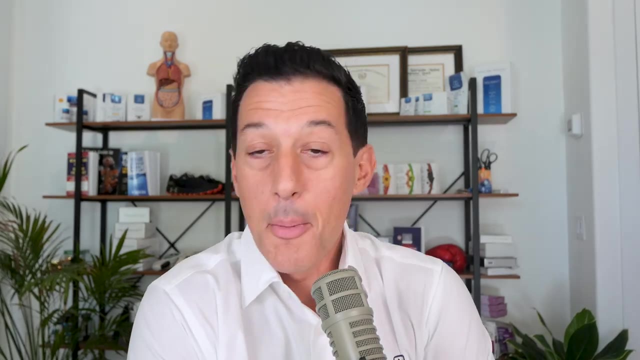 I've talked about different brands before. We can try to link up these for you. at stephencabralcom forward slash 2477, which is today's show notes. Cadmium, also found in drinking water. I've shared that before, but also, like a lot of it, is environmental based batteries. 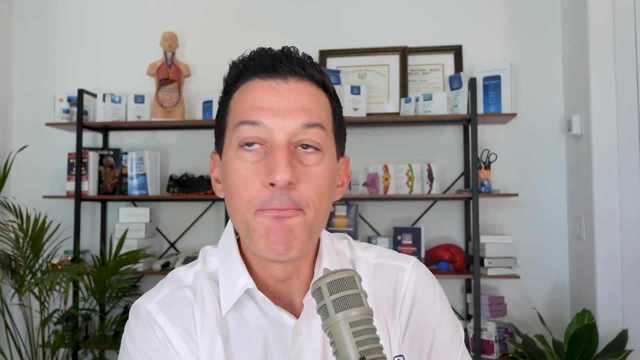 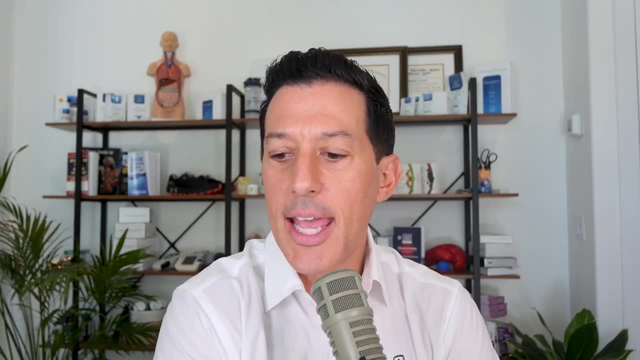 certain pigments and so on. So it's a lot of different things. So it's a lot of different and colors and paints not really airborne, not really fume wise unless you're working specifically with it. Some plastics- for the most part, that's where you're going to get it, But also 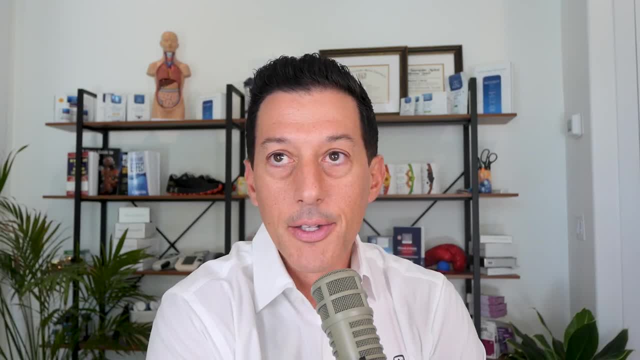 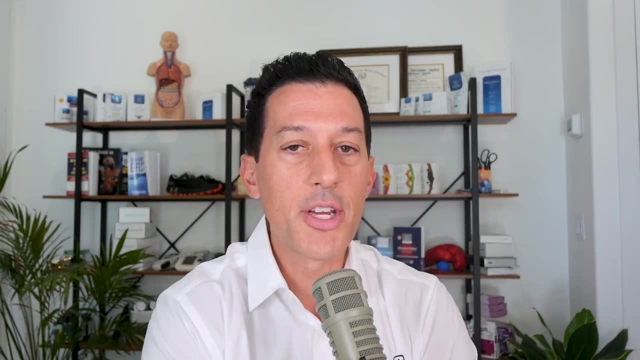 you have to be careful with things like mushrooms, and even like crustaceans or shellfish or even algae, because these things will often be present at that, especially mushrooms. You want to make sure your mushrooms are tested for no heavy metals, not even just food-based ones. but if 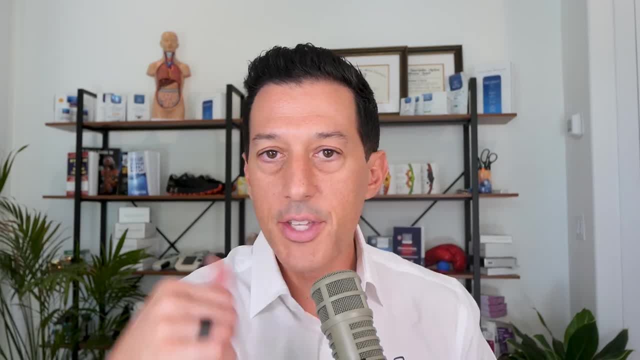 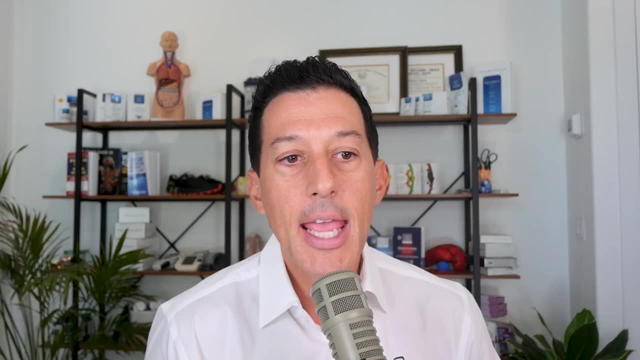 you're taking mushroom-based supplements as well. All right, lead. This is from Older, Old Homes. Remember old pipes? water still runs through lead pipes in many, many cities and towns, And so that's something to watch out for. So water from your old pipes and then lead paint. 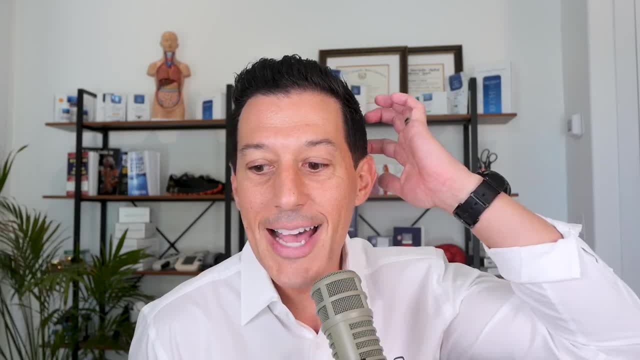 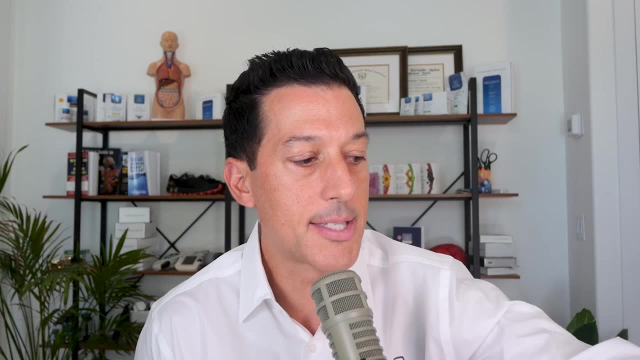 et cetera. So those are the main ones that we're going through. Mercury would be the last one. Mercury, oh, it can be from everything, from what's the best way to say this, so I don't get banned Again, I'm not saying to do it or not do it, but certain shots It can be in light bulbs. 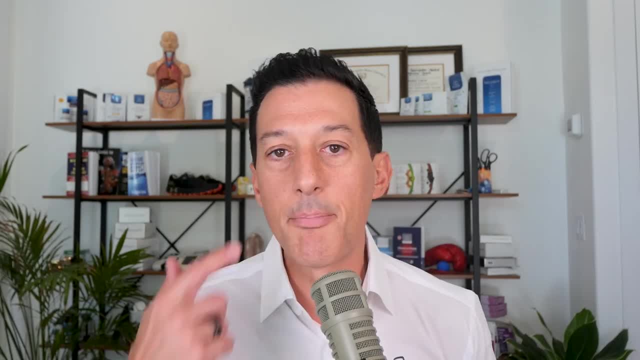 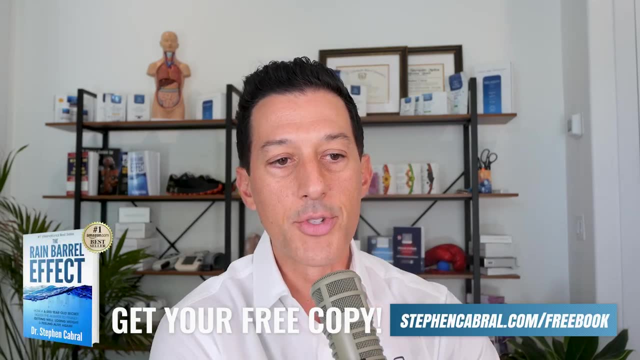 It can be in old thermometers, But mainly it's from fish and dental amalgams that I talk about in my book, The Rain Barrel Effect. So you have to be really careful. Don't have your mercury amalgams, your silver fillings. 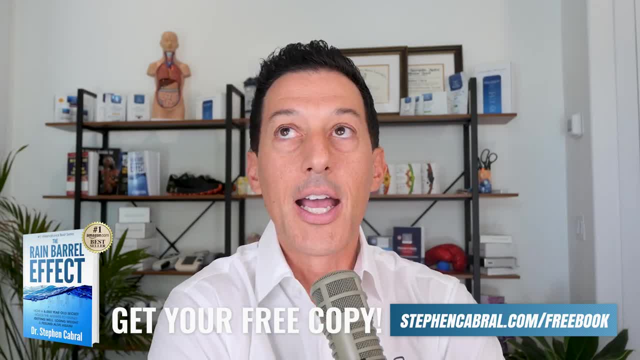 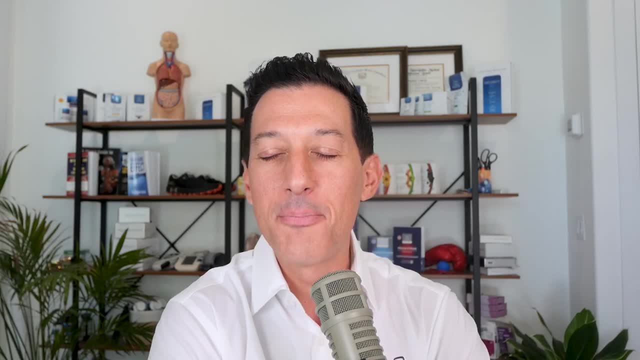 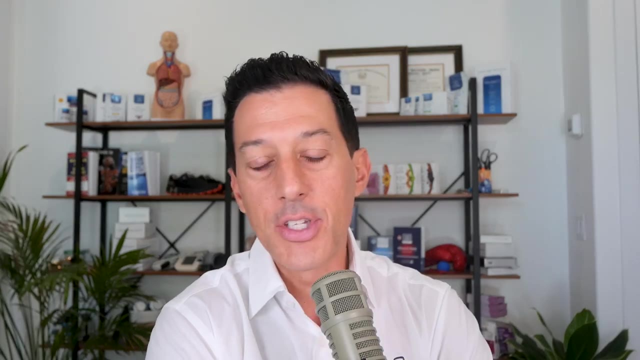 taken out by a regular dentist. Make sure you're going to, and the organization is called IAOMT- I had to memorize that IAOMTorg- And you'll be able to find a biological dentist there that can do a true extraction as needed. So that's that, And definitely again follow a heavy metal detox. 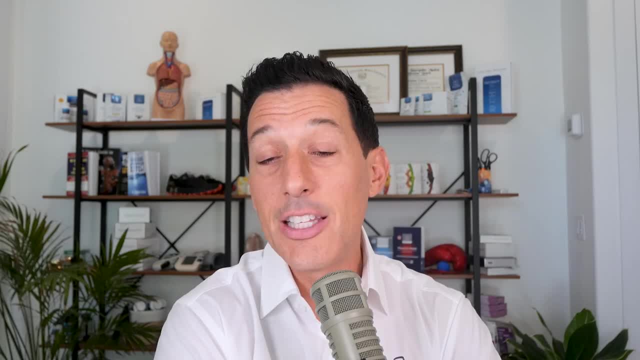 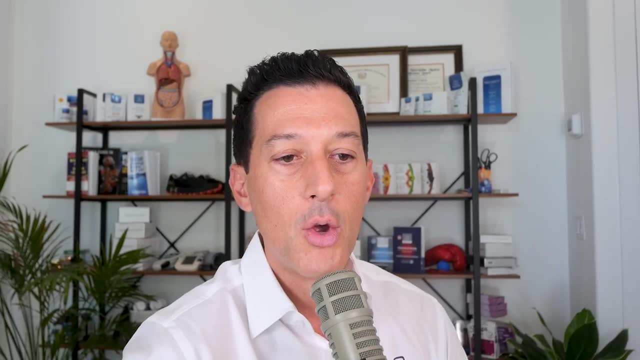 use infrared sauna if you're going to have them removed, but eat low mercury-based fish- Really, really important, And I have a whole podcast on that, So we'll link that up today too. at stephencabalcom forward slash 2477.. All right, but let's get into. how do these heavy 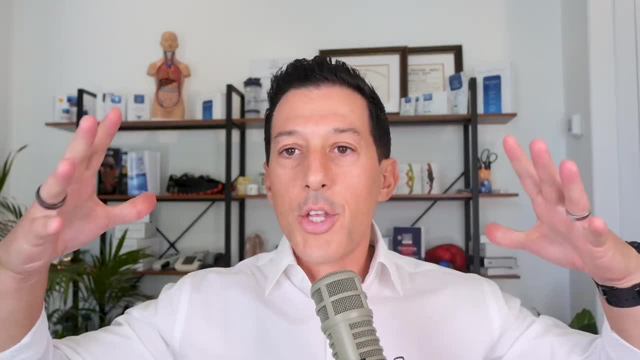 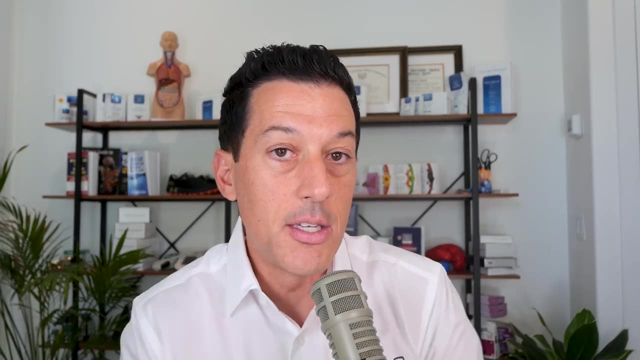 metals now affect the gut. Well, what happens is this: The heavy metals are consumed with the water or the food And when they come into our gut, which is about 26 feet of digestive lining from the start of the mouth all the way through the stomach, they're going to be consumed by the 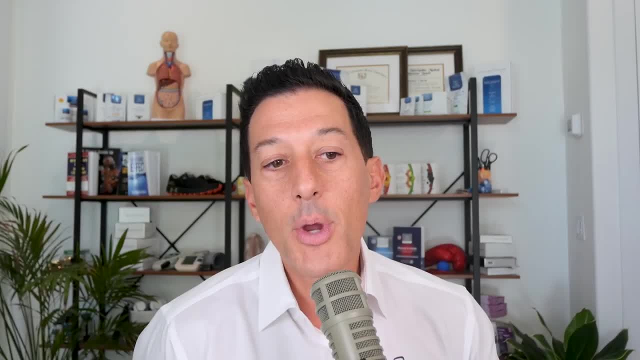 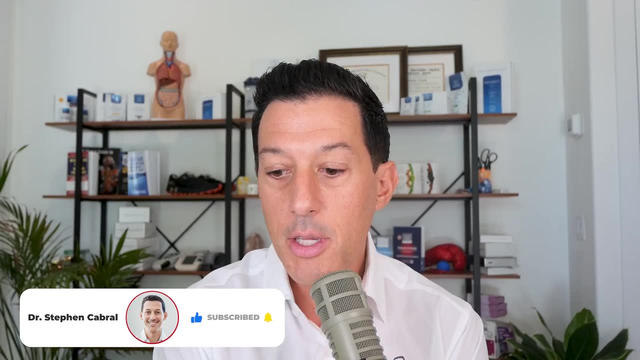 stomach, and then through the small intestine, and then through the large intestine, And what happens is they begin to. not so a lot of it will be excreted, There's no doubt about it- but some of it will actually begin to lodge and get mixed in what's called the intestinal epithelium. So that's. 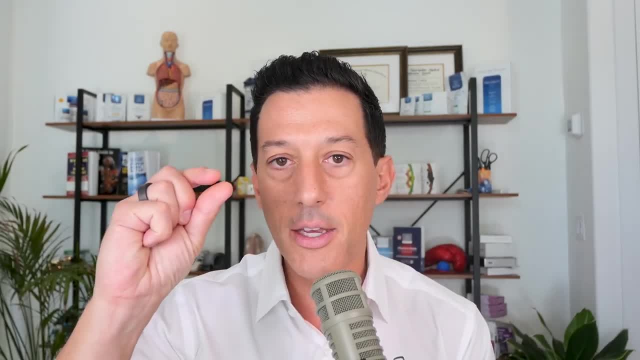 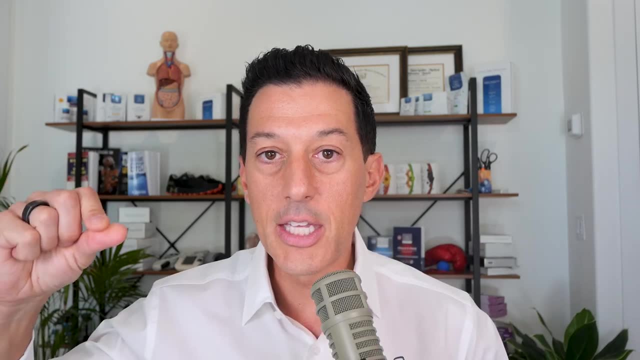 basically the lining of your gut And, believe it or not, it's very, very thin. It really is, And so when you look at that, the heavy metals begin to interact with the bacteria there. They begin to be used to create biofilms- And I've talked about biofilms a lot, but they're 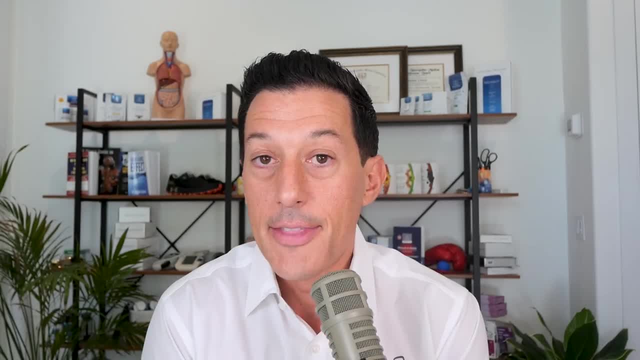 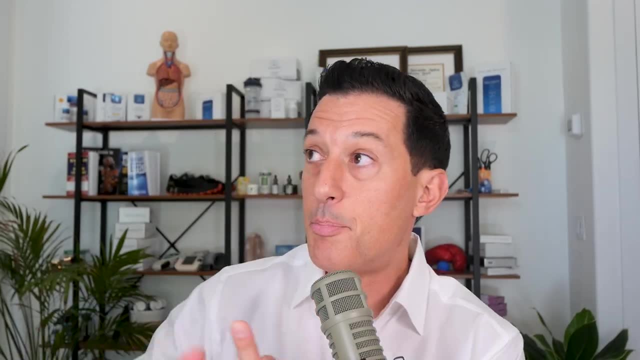 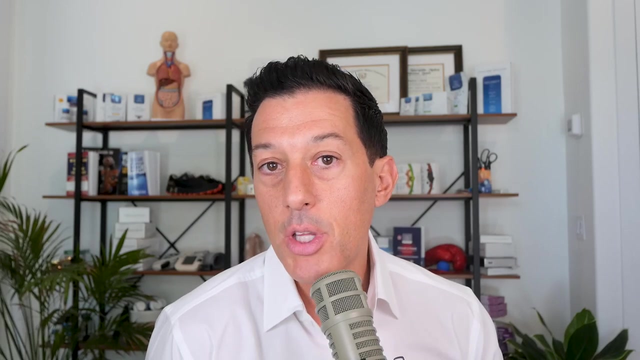 biofilms before and how they can be very dangerous for your body. They don't allow them for proper absorption, So you're oftentimes not making the iron that you need, the B12 that you need, What else- Vitamin K and many others- So just keep that in mind Really, really important. 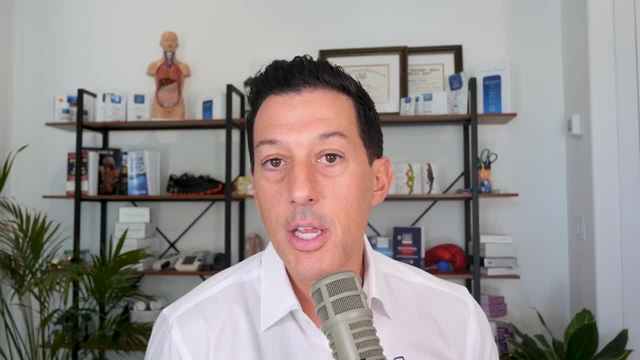 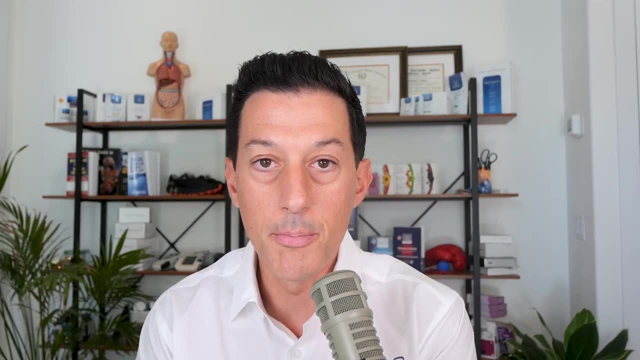 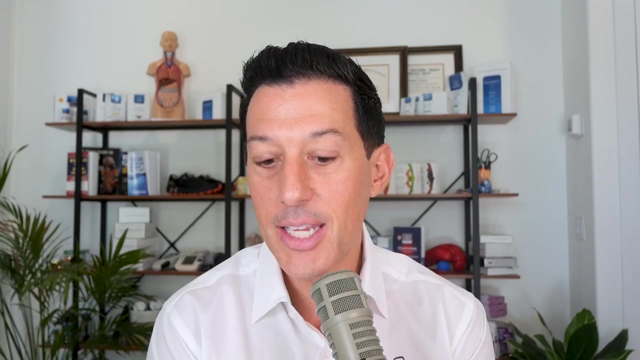 But one factor I think that often gets overlooked is it creates oxidative stress, So it creates inflammation, So your body knows that that metal shouldn't be there. There's an immune reaction And what happens is that inflammation is created. Now, when inflammation happens, 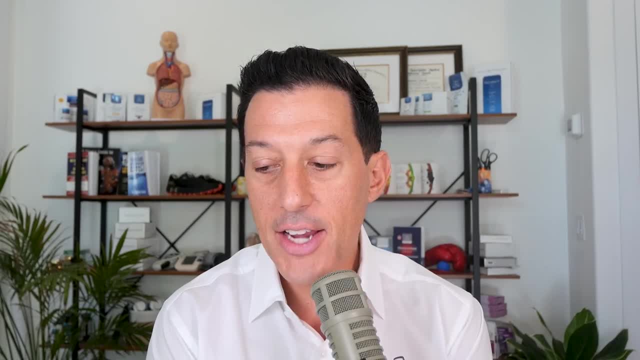 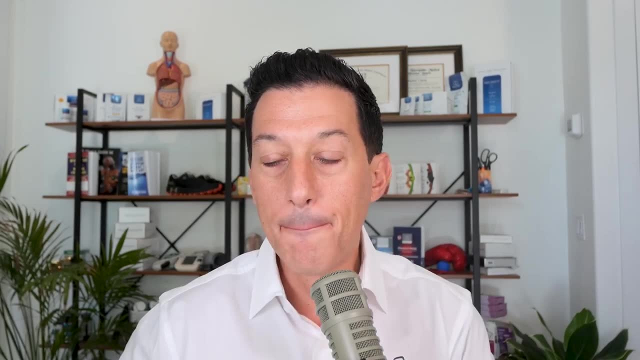 it can affect the actual bacteria in your gut microbiome. It can affect your absorption of certain vitamins and minerals. It can cause water retention, gas pain, bloating, but it can also create intestinal permeability. So now we have these heavy metals that were contained inside. 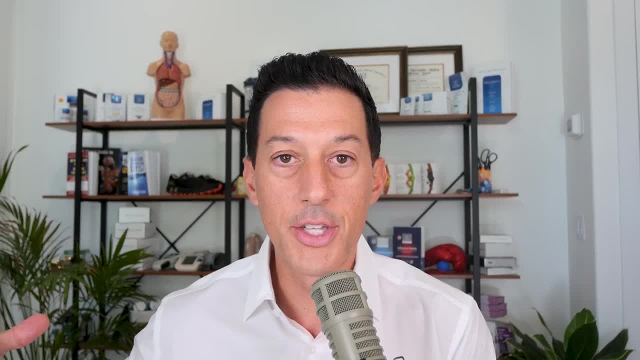 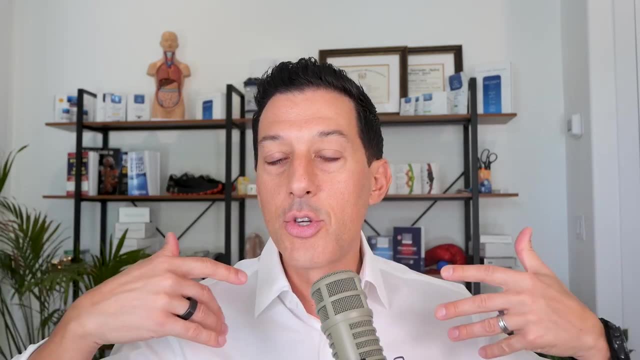 your digestive system that are now starting to move out into your bloodstream. All right, So now they seep out through your bloodstream of about 20%, 26 digestive tract And they can go now to anywhere- The brain, right, Alzheimer's. dementia. They can go to your liver. They can go to your thyroid for things like Hashimoto's. They can go to your joints for things like rheumatoid arthritis. They can go to where Nervous system for MS, for overall in the body, lupus, fibromyalgia, et cetera. So again, let's keep in. 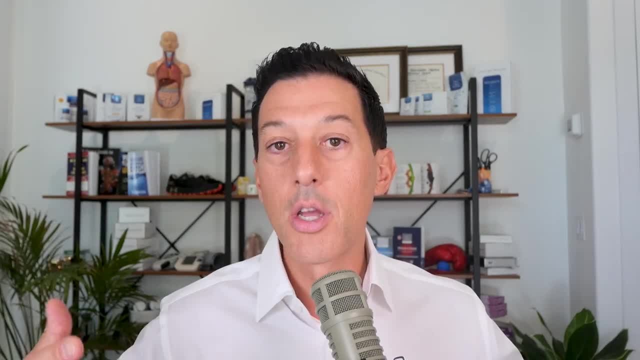 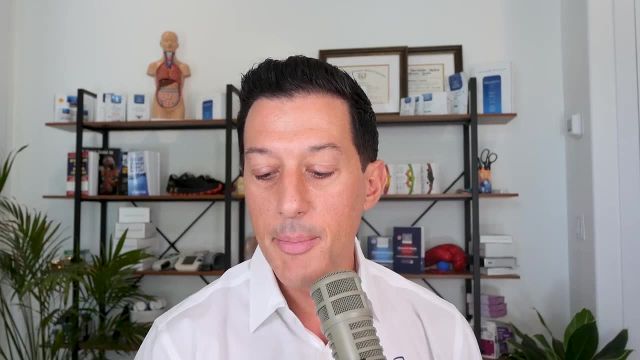 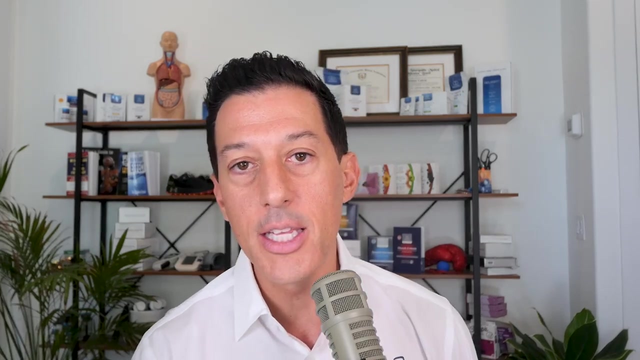 mind that heavy metals can be an underlying root cause of autoimmune issues or things like migraines from inflammation, Psoriasis- which is autoimmune as well in many cases- skin conditions et cetera. So that's worst case. Then it starts to move into the body, because now we need to eliminate these. 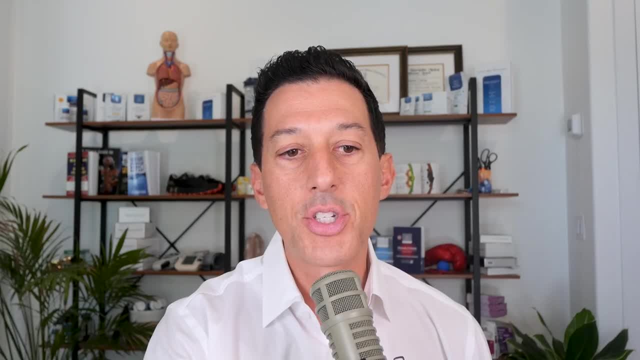 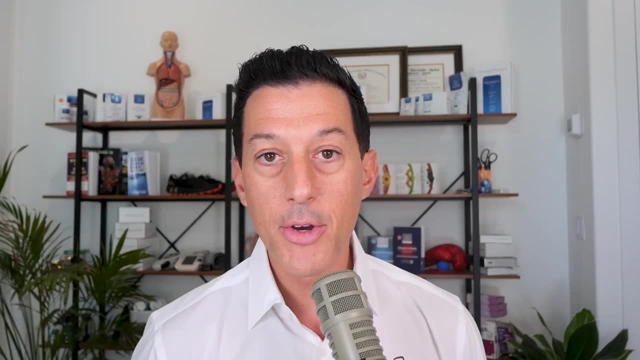 from the body. So really, really important that we look at that, but just understanding that we have a root cause: heavy metals being consumed, causing damage to the gut microbiome. now poor absorption of vitamins and minerals, So we lead to deficiencies, And then these metals. 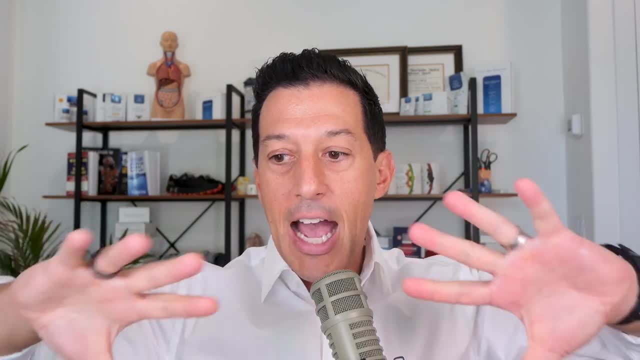 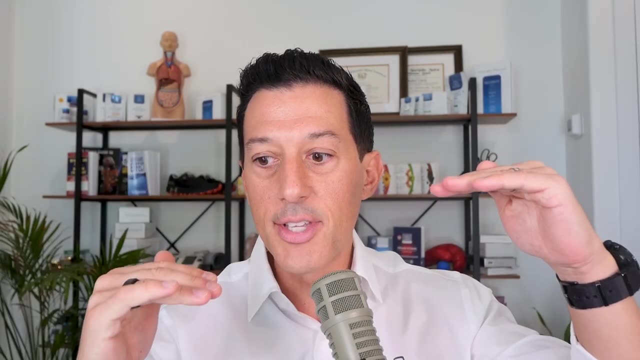 get into our bloodstream, which is toxicities, right? So when I talk about how do you heal? Well, healing is an equation, So it's bringing up your deficiencies and lowering your toxicities. Well, in order to do that, we need to remove the heavy metals and then we need to rebalance the 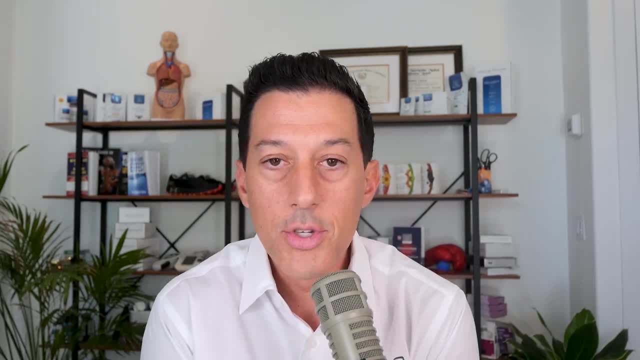 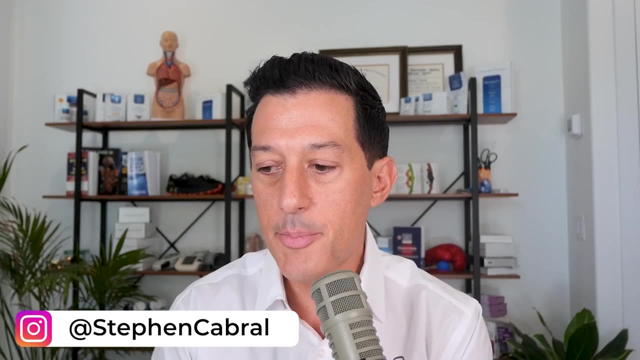 gut microbiome And you can do that right. So once you know how to do this, then that is the healing process. That's how you begin to empty your rain barrel. So, of course, as you're doing something maybe like the CBO protocol and the CBO finisher, or, let's say, like the heavy metal, 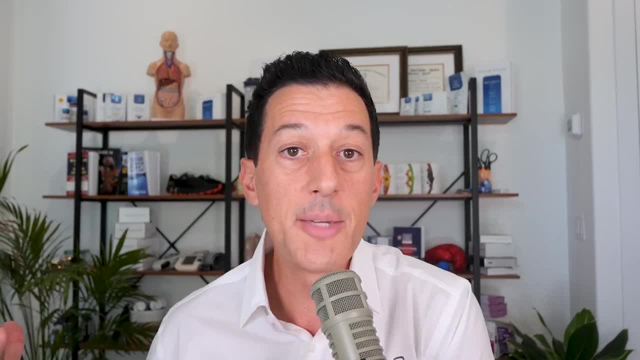 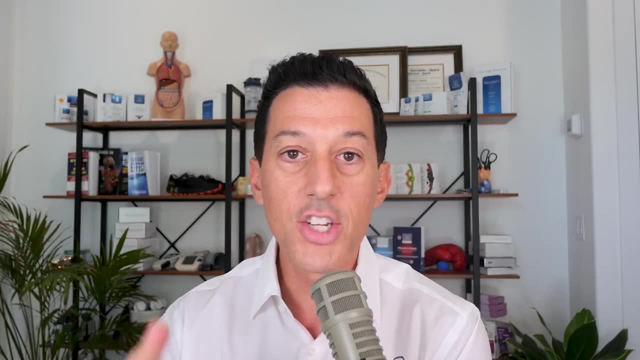 detox, or in the functional medicine detox, or whatever you might be doing, do keep in mind that you have to then limit the new intake of heavy metals. So you're using a water filter, right. You're using a shower filter, let's say, or bath filter for your kids or yourself. 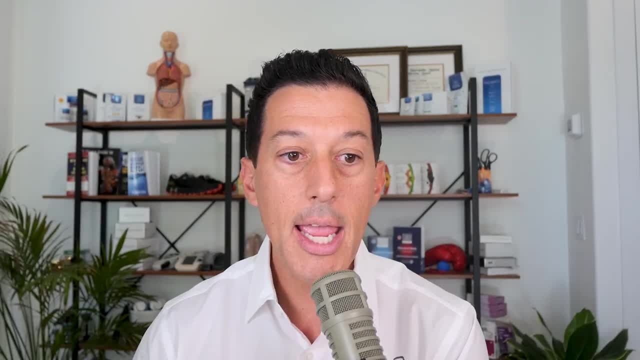 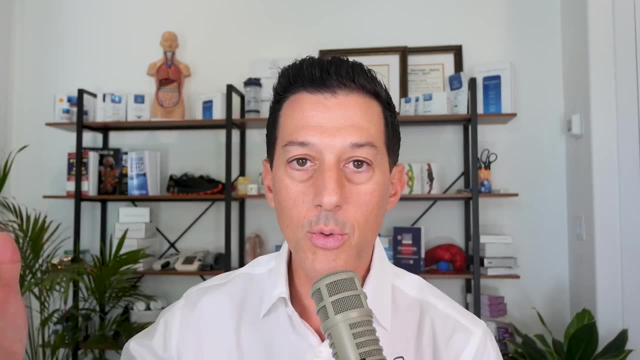 You're going to eat low mercury fish And you're going to make sure, if you have rice, that you're having low arsenic-based rice, and that's how you do it right. You're going to start to switch out your pans, your cooking ware, over time. Again, all these resources are at stephencabralcom. 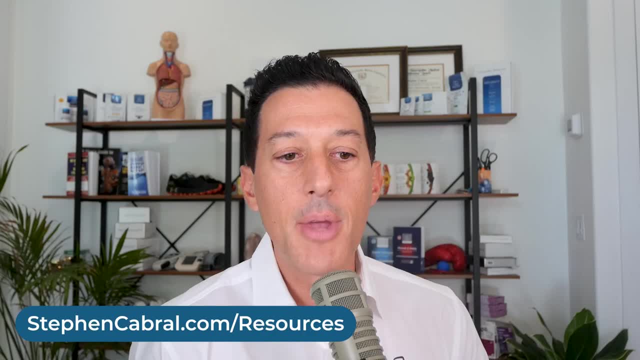 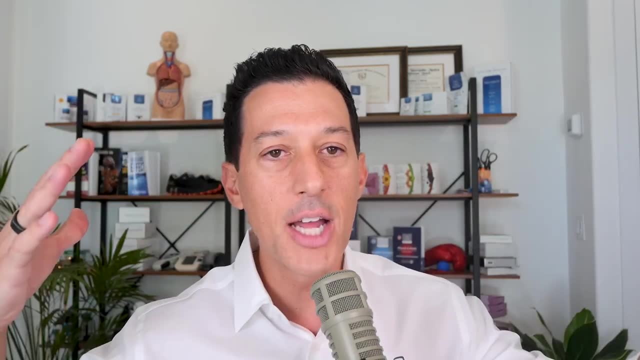 forward, slash resources, literally over 100 different companies that I recommend that I use with my own family, And this is really, really how we begin the healing process. So I'm not going to go over rebalancing the gut today because I have lots of podcasts on that. I have a whole category podcast just on digestion. So 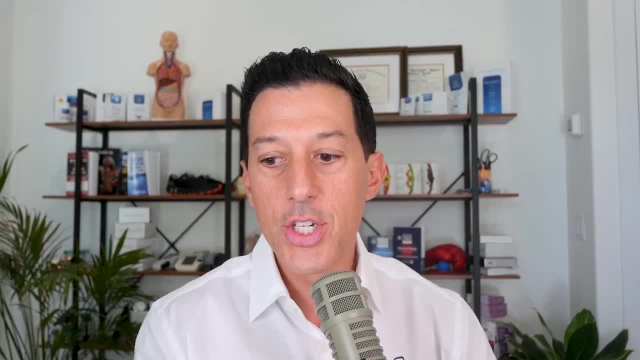 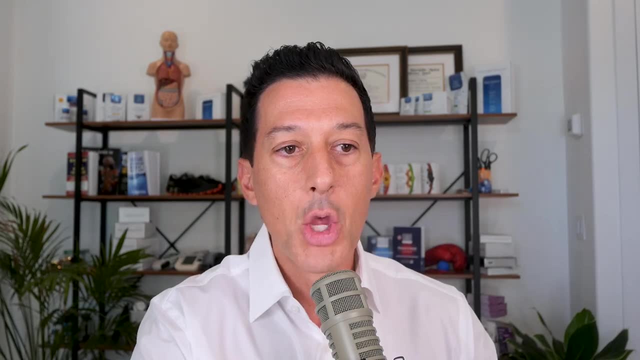 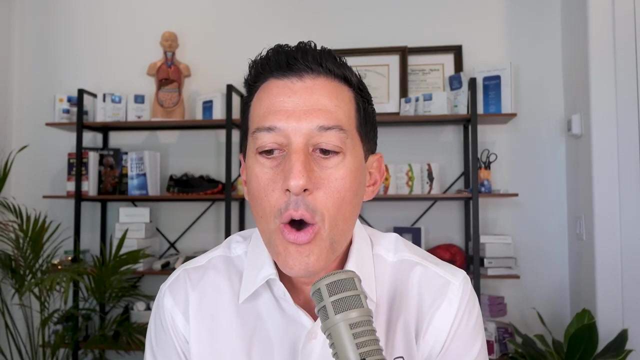 again. we'll link that up today at stephencabralcom forward- slash 2477,. stephencabralcom forward- slash 2477.. But I just want you to understand. so I'm not going to make this a long show, because what I want to do is just try to impress upon you of how disease is created in. 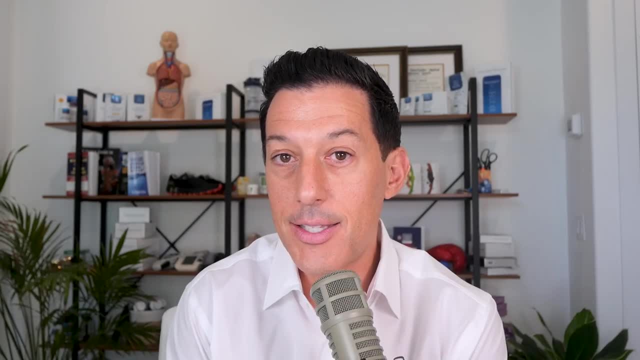 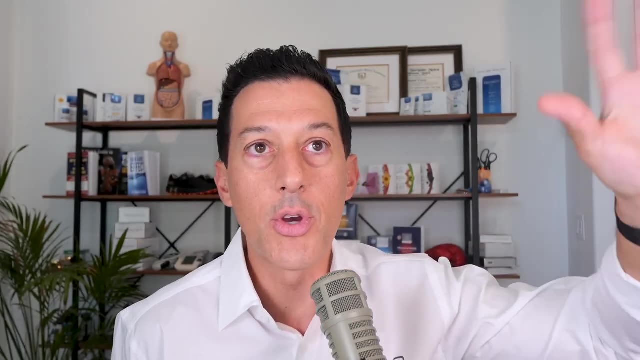 the body, but also how. How dis-ease right A dis-ease of the body can also be reversed. Okay, So let's say heavy metals was the cause. You were drinking water. you didn't know that had aluminum in it, Then you're using. 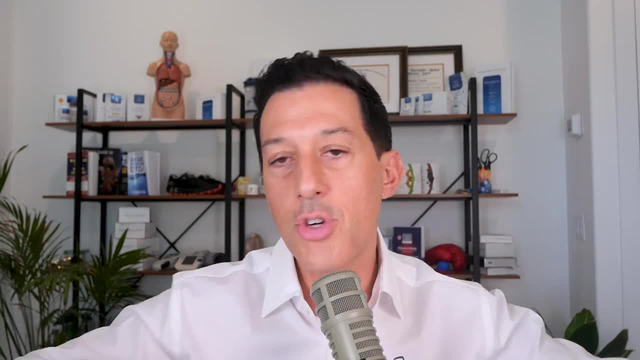 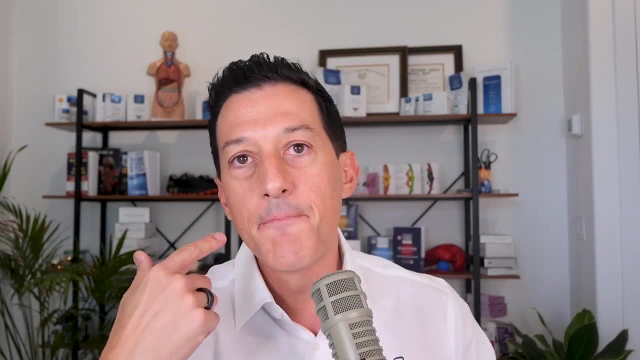 aluminum deodorant. and then you have aluminum pans with a metal spatula and you're scraping those pans every time and you're getting a little aluminum in your food. And then you're using aluminum foil and then, over time, these things begin to build up And then you've got mercury. 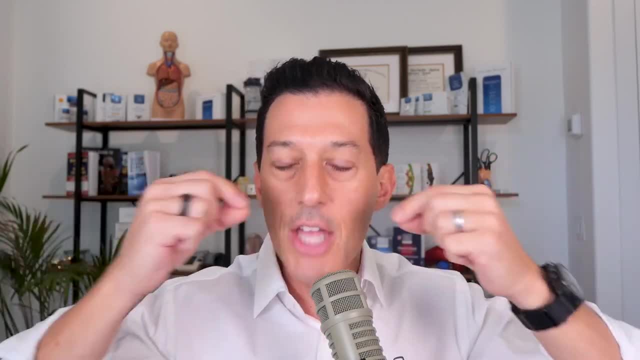 amalgams in your mouth. You've got like four of them and they're 20 years old and the edges are starting to turn up. I talk about them a lot but they're not going to turn up. And then you've got. 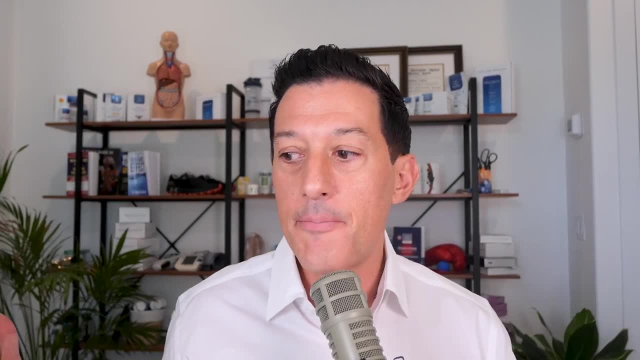 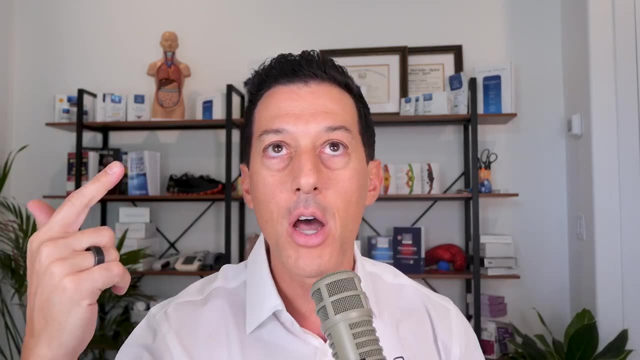 my book And then all these metals are now in your body. Now you're 48 years old and you've got the early signs of high blood pressure, high cholesterol and an autoimmune issue And you're like: how did this happen, Right? Well, okay, Now you might also have some bloating digestive. 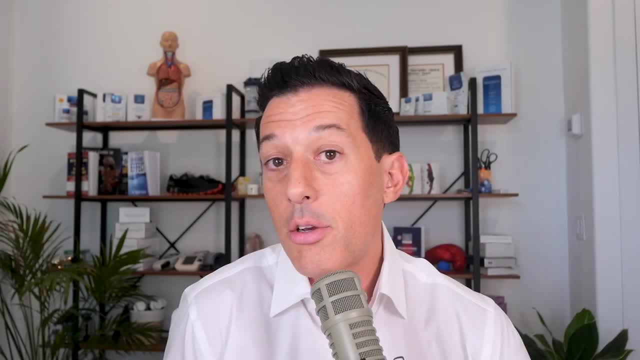 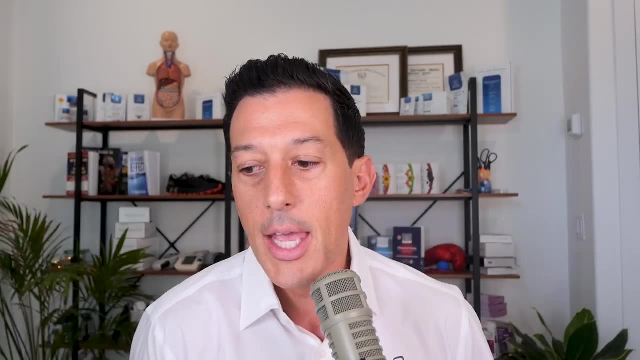 issues as well: poor bowel movements. This can start, believe it or not, with just higher levels. We always see- Not always, but we see- elevated levels of aluminum, and secondarily we can see mercury, And so, again, I'm just sharing with you exactly what's going on, And then you have 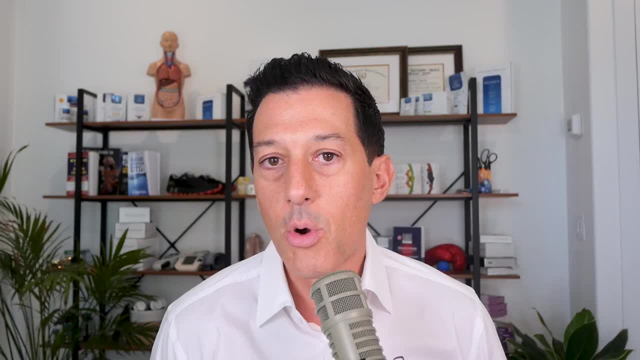 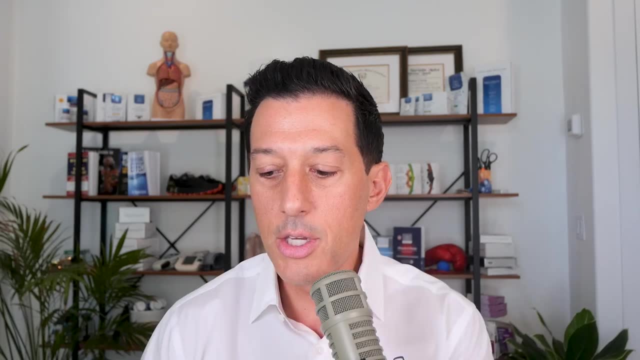 what we find in clinical practice, And so that doesn't mean that it's the end of the world, And it certainly doesn't mean that you need to have high blood pressure, high cholesterol or an autoimmune issue for the rest of your life. You don't. What we need to do is first go through the 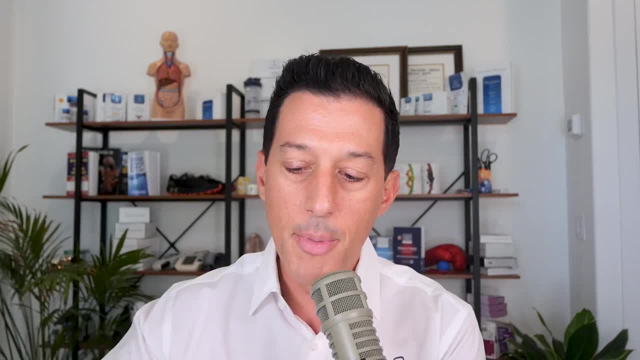 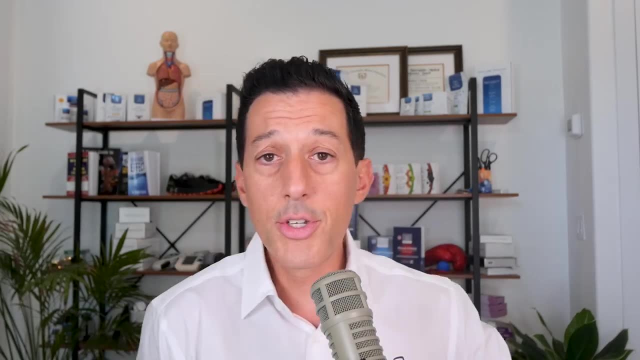 process right, So, again, I can't provide. I just have to give you the disclaimer: no medical advice, no medical cures, no medical diagnosis, or no medical- What's the other one? Treatment plans. There we go. So what we're going to do, though, is rebalance the body right, So we're 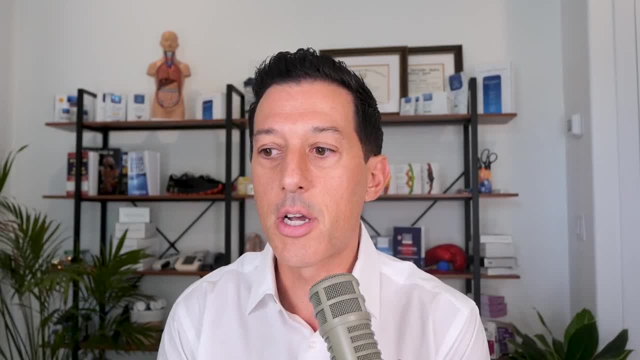 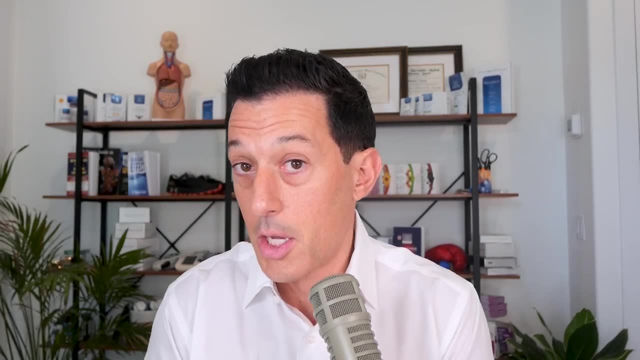 going to, okay, open up detox pathways, 21-day functional medicine detox, start doing infrared. what are we going to do next? We're going to then move into some type of gut healing program, like, let's just say, the CBO protocol, And then, either at the same time or after, we're going to 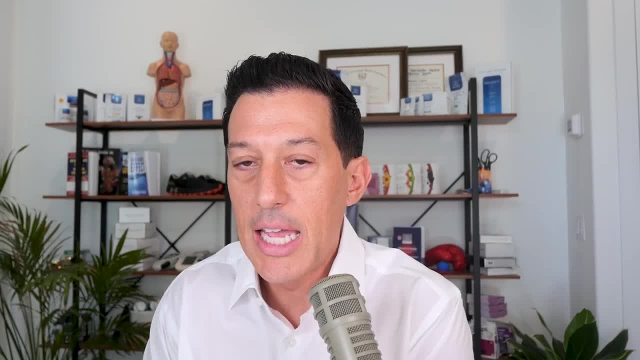 do the heavy metal detox, because we might as well get these metals out of our body but also don't put more in at the same time, and we have to seal that gut right. So that's part of the CBO finisher. 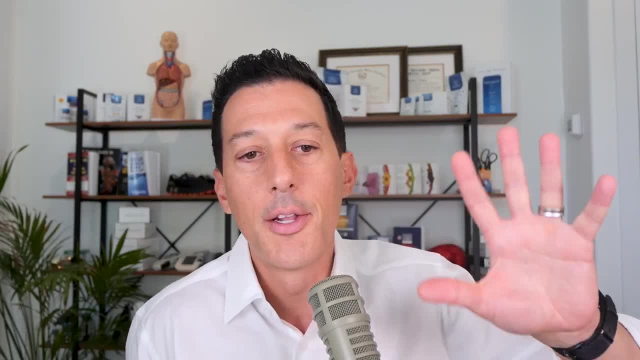 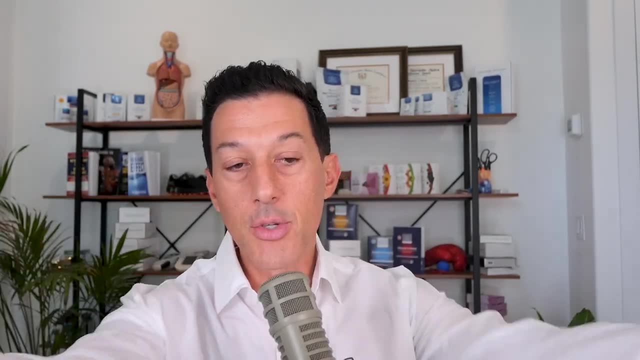 So I'm not going to give you like step-by-step today because, again, I don't want to glaze over this. It's too important to glaze over. It really is What I would do. you can actually run this lab very, very easily with a little bit of snips of.